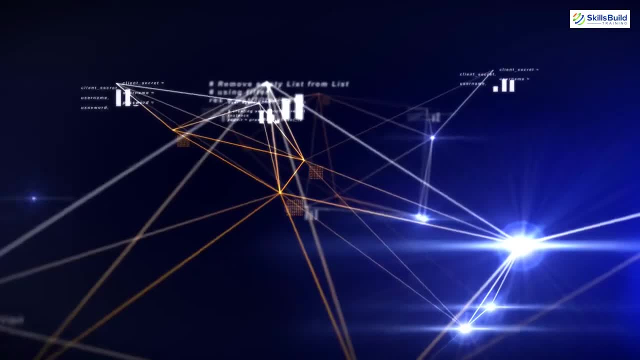 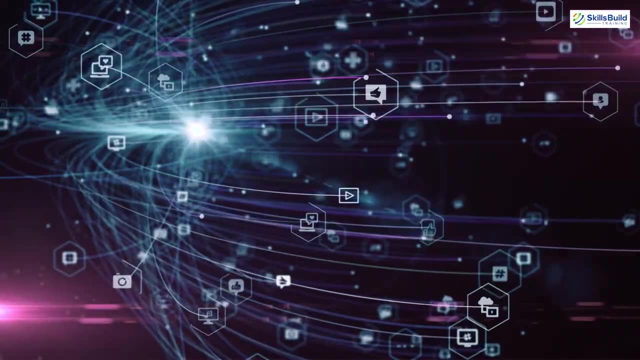 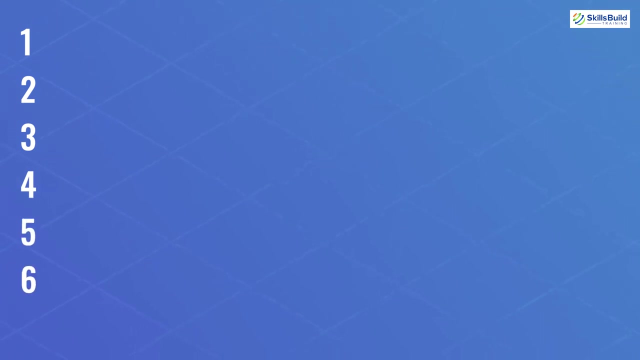 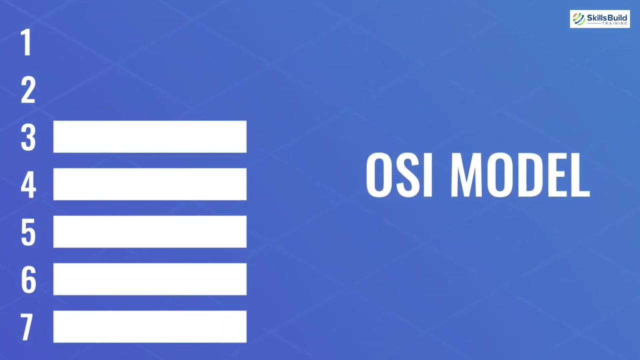 like that: when we transfer something on the internet, it passes through some protocols, take some paths and follows some guidelines in order to reach a destination system. basically, we have seven layers on the internet through which the data have to pass through, and those seven layers are called. it look something like this: at the top we have application layer and then we have presentation. 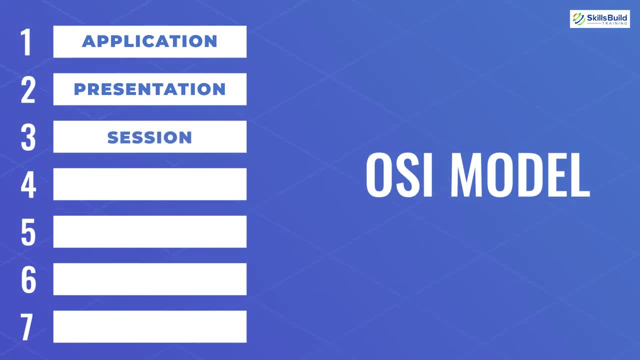 layer, and then we have session layer and it follows transport layer, and then we have network layer and second last layer is data network layer and the last one is physical layer. well, there is no universal rule that which layer is the first one and which layer is the last one, because, if you are, 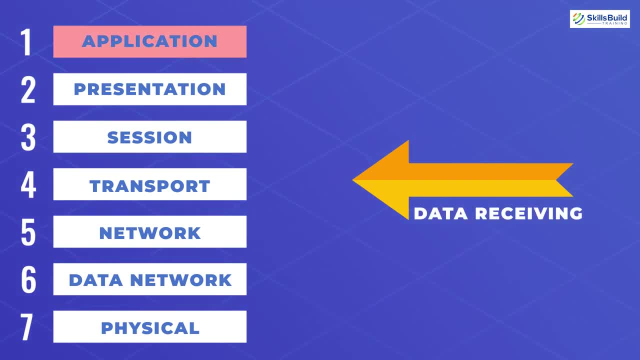 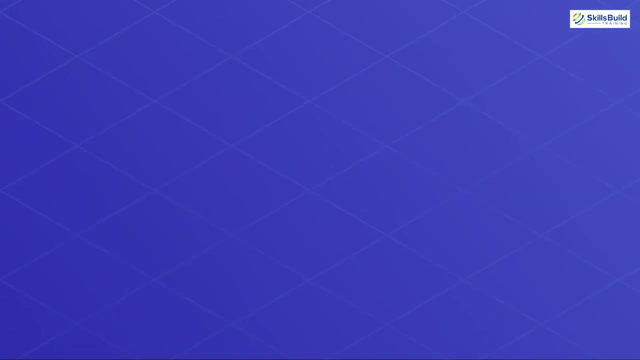 sending data, you might see application layer as the first layer and if you are sending the data, you might see physical layer as the sending layer, or it can be vice versa. so it all depends that how you conceive this and how you understand about it. let's have a little introduction about what each 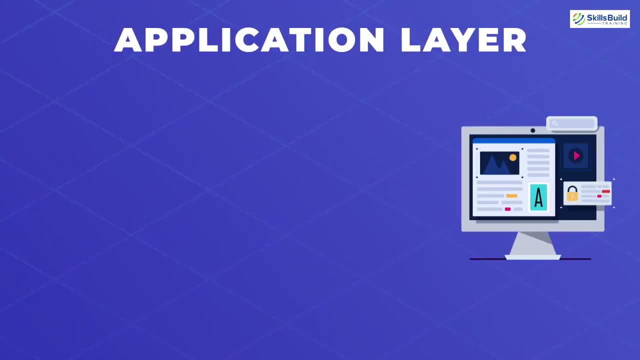 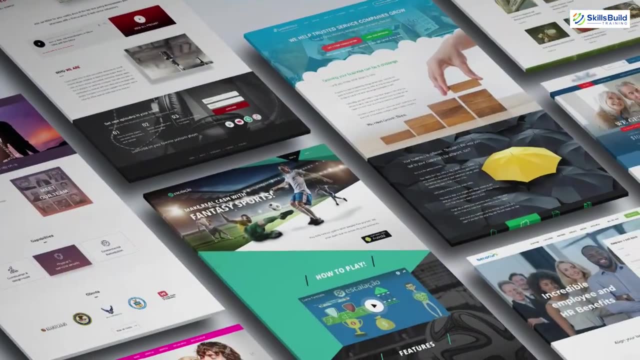 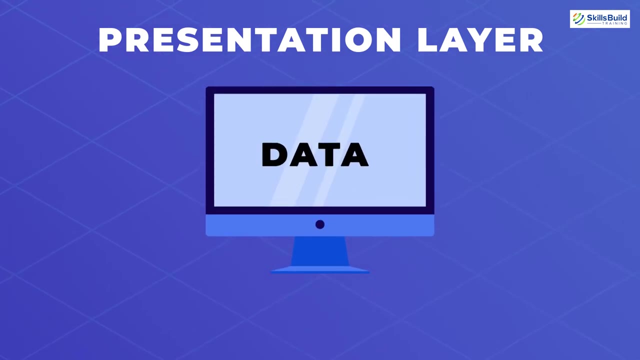 layer performs. the application layer is your end device or your software, like your web browser or whatever you see on the screen is basically is on the application layer. the presentation layer prepares the data. it means the data which is to be shown on the application layer. it also defines. 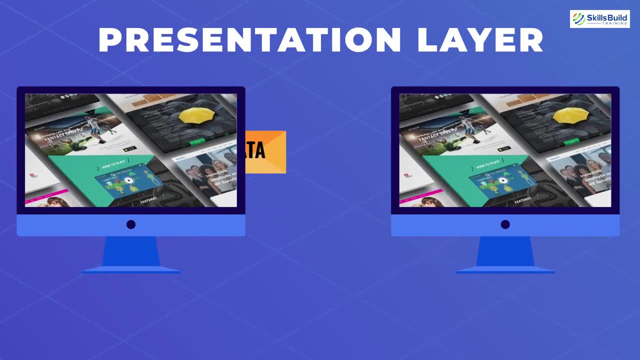 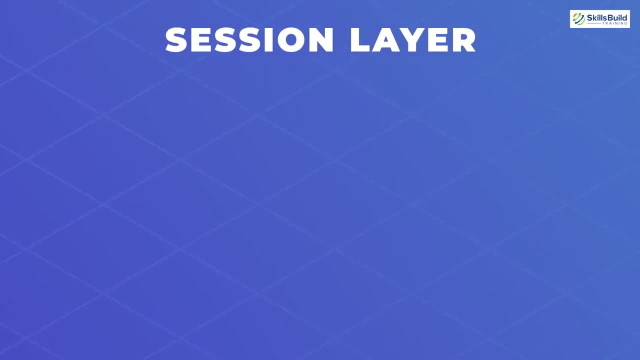 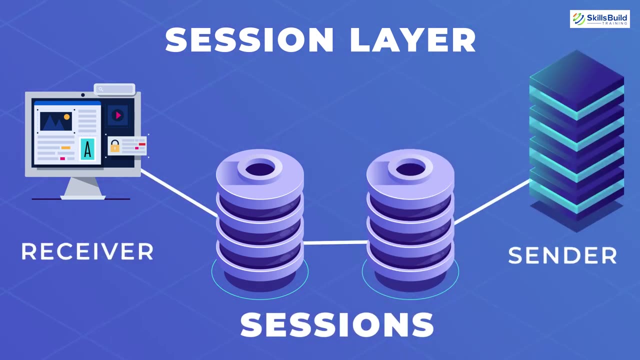 that how two devices should process the data so that it can reach the destination correctly. the next layer is session layer and it is responsible for creating the communication channels, and they are known as sessions. we create these channels between the sending and receiving devices. the next layer is transport. 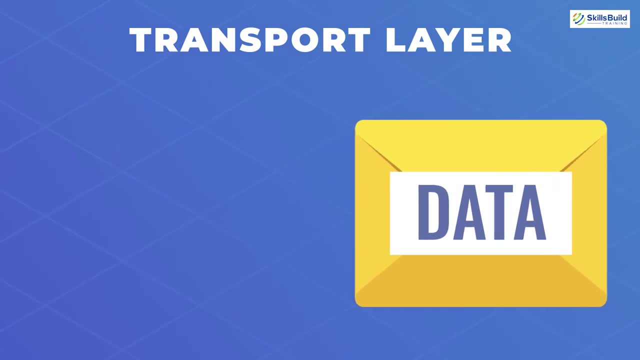 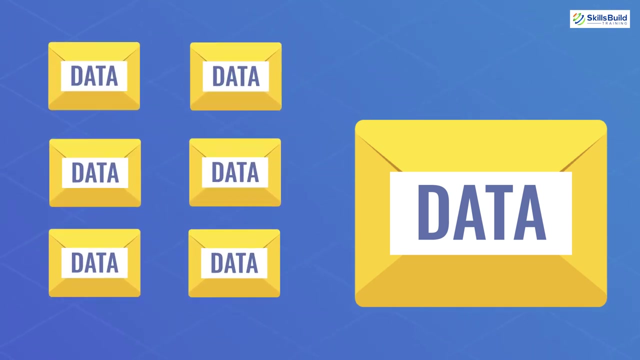 layer and it works on the data, the data which gets transferred to the session layer and breaks it into segments. in simple words, by segment we mean small pads. it is also responsible for assembling the segments when it receives the data. the TCP protocol works on this layer. so, obviously, when we divide a 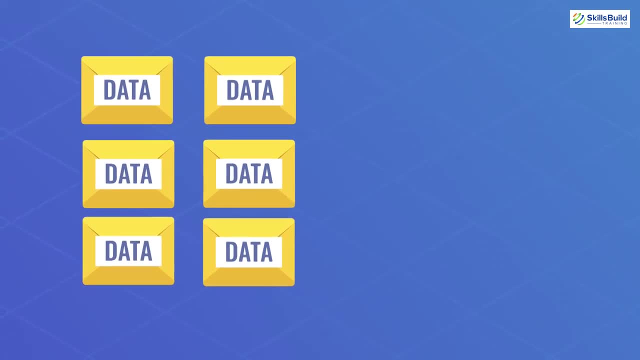 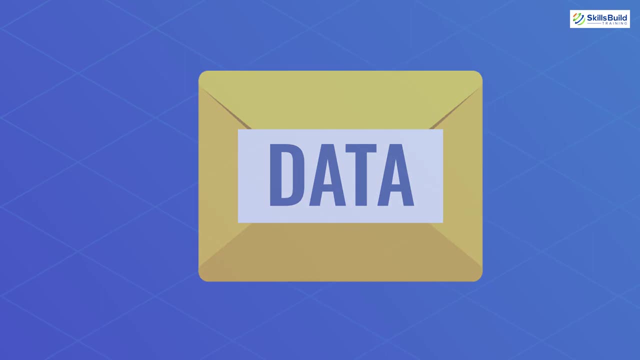 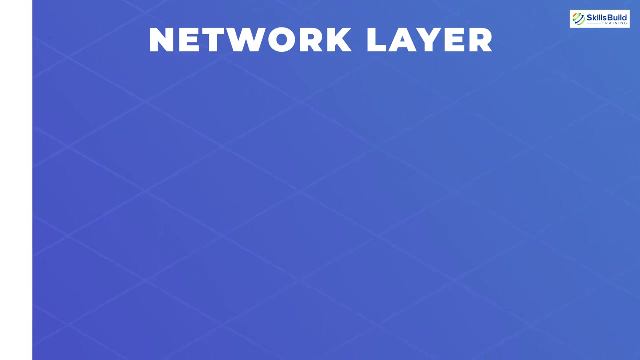 data or a data into segments. we must reassemble those segments in order to get the data in full form. transport layer work on that. the next layer is network layer. basically it has two functions. the first one is to break the segments which we got from the transport layer into the network. 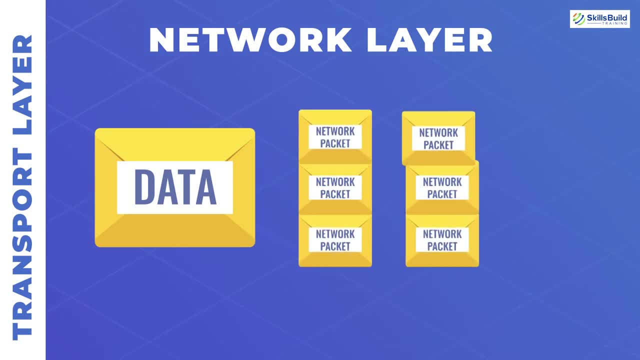 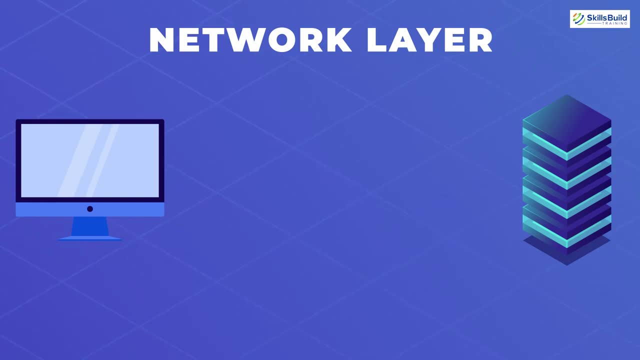 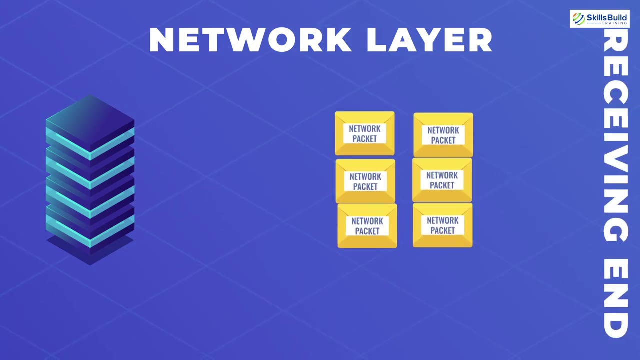 packets. so it means we will divide the data in more smaller pieces. basically, the data which travels into the network travels in the form of packets. the second function of the network layer is to reassemble those segments on the receiving end. the IP protocol works on this layer. the data. 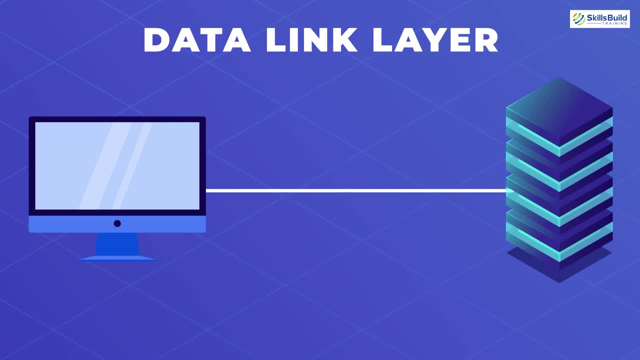 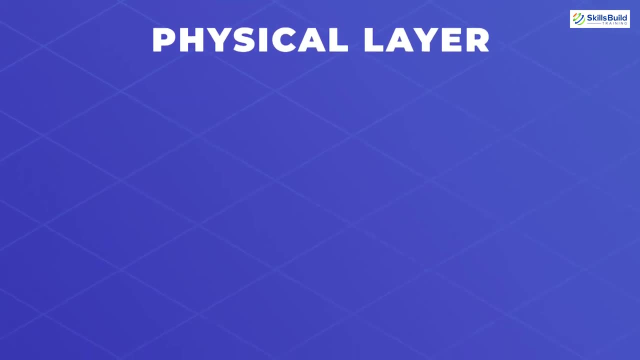 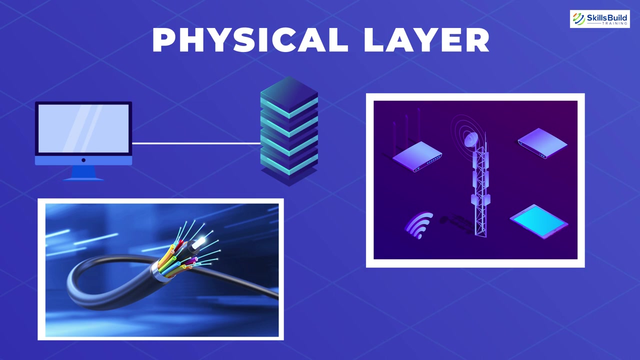 linked layer is responsible for establishing and terminating the connection between the two nodes which are connected physically. the last layer, which is known as physical layer, is responsible for physical connection network nodes, and it can be through some physical cables or through a wireless network. in modern day internet, both means of connection are getting used. so that was all about the osi model and 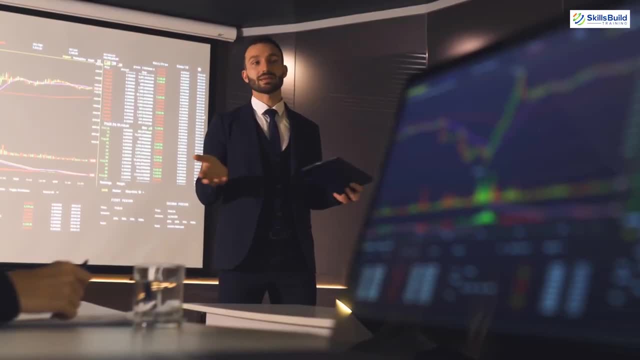 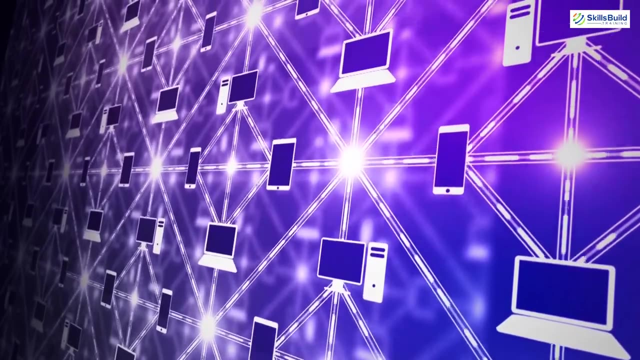 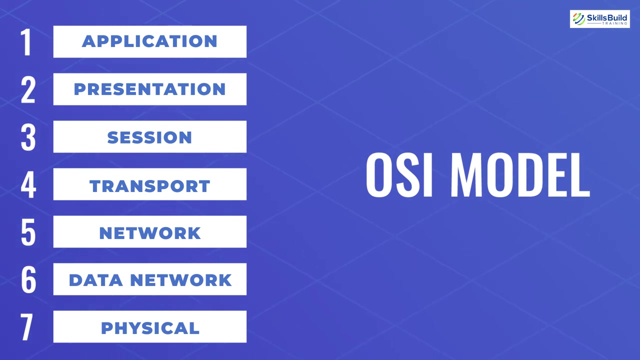 if you want to understand how it works, please let us know. we will have a brief video on that by now. we know that- how our data gets transferred from one place to another and what are the layers and their responsibilities involved in all of this operation. now let's talk about the tcp ip. 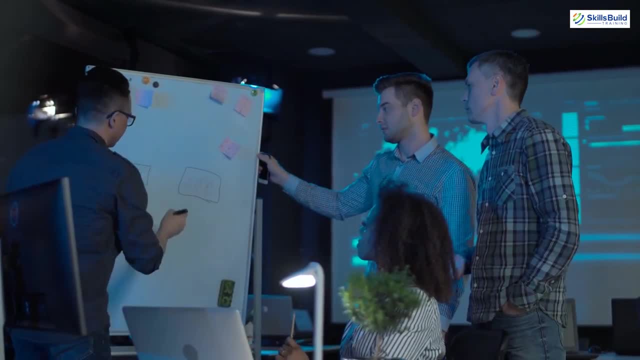 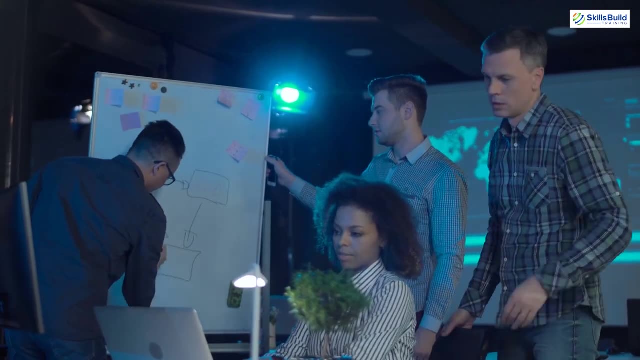 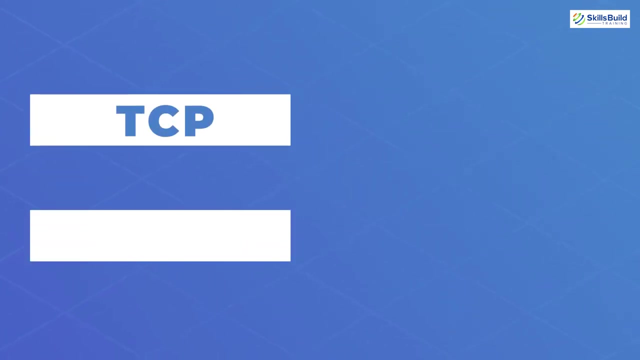 most people take these two as single unit because they are often called together, just like we are calling them together, and that is why people get it wrong to think of them as single thing, but in reality they both are different. they work on different layers too, as i have told you earlier. 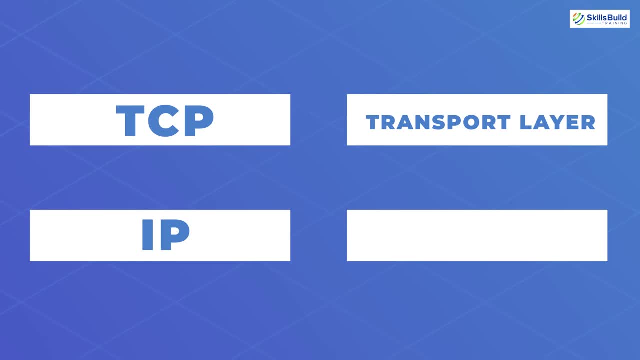 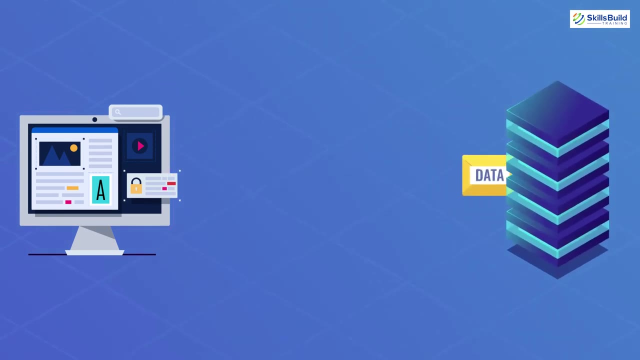 that tcp work on transport layer and ip works on network layer, so let's see how they differ from each other in terms of their functionalities. the tcp protocol is responsible for the delivery of data towards the destination which gets sent, and it sends the data towards an ip address, and 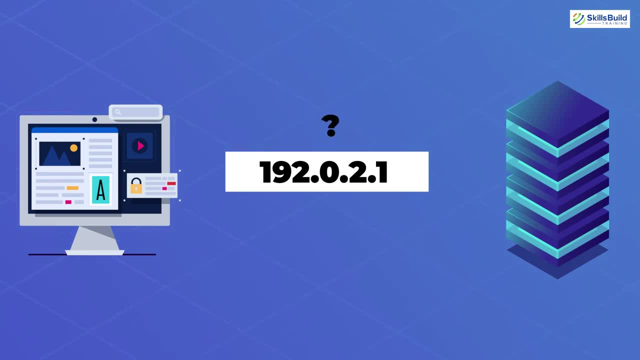 from where does this ip address comes from? that is the question. this is where ip comes in. ip protocol is responsible for obtaining the ip address, and then tcp protocol uses that ip address to send the data to that ip address. so it means they both are dependable upon each other somehow. now the question is why they are often. 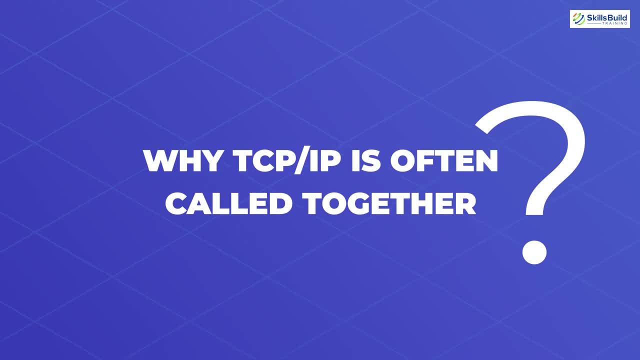 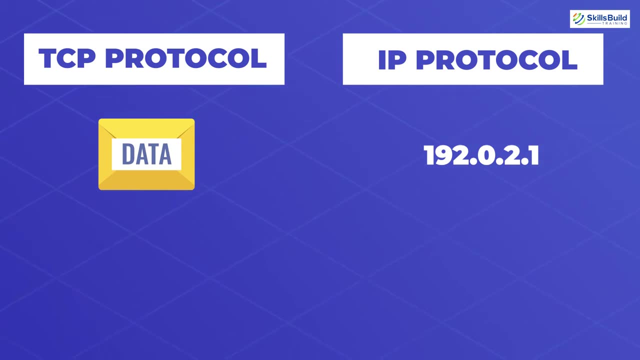 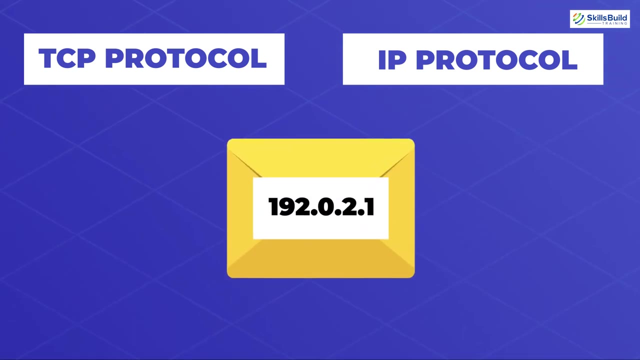 talked together when they have different jobs to do. well, it is possible to differentiate them on the basis of their job and the work they perform, but as they both get used together, that is why many people take them as single entity. if you take a daily life example to understand it. in more, better way. just think of a phone number and think of it as your ip protocol and the tcp protocol is like the technology in your phone which makes your phone ring and helps and allows you to talk to another person on another phone. yes, their duties and work is different. 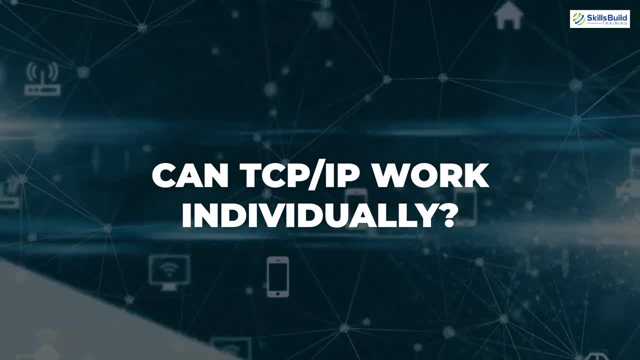 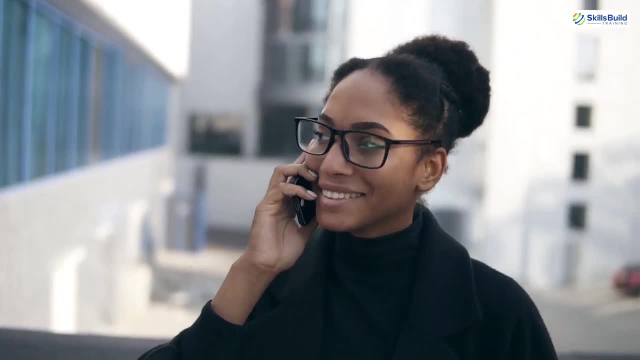 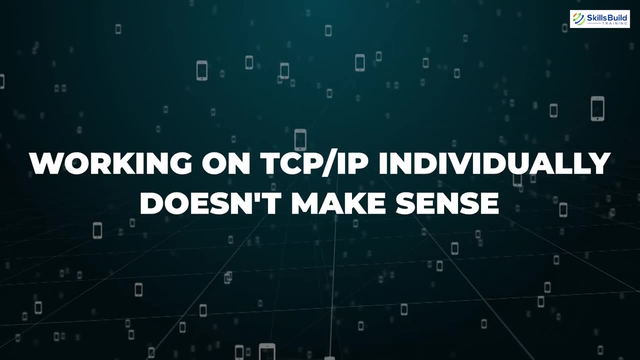 but would it be possible for both of them to work individually? obviously your phone number needs a technology to make it work in more efficient way. obviously, if we differentiate them and we try to work them separately, that would be meaningless. and now let's see how tcp ip work in. 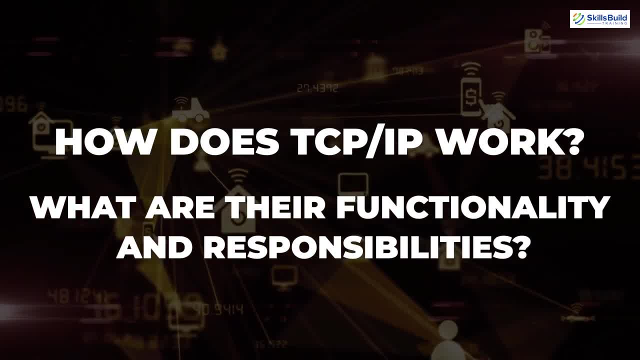 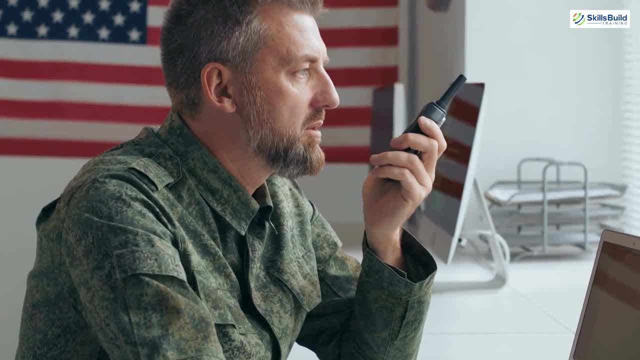 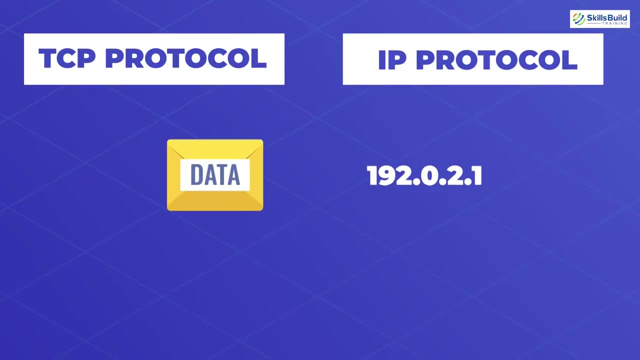 detail and let's see what are their functionalities and responsibilities. the origin of tcp ip took place by the us department of defense to define that how the data will get transferred from one device to another. tcp ip defines that how the data will be exchanged over the internet. 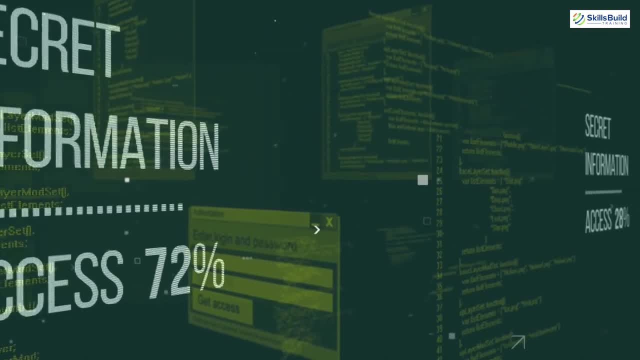 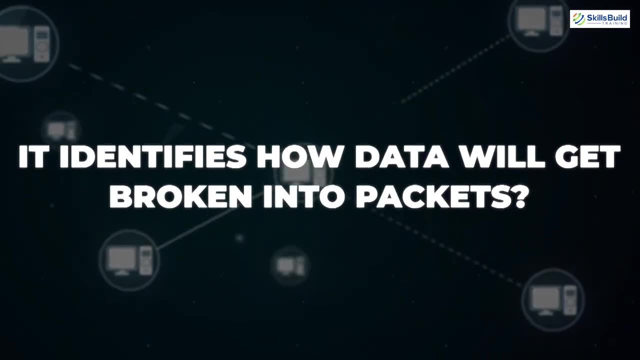 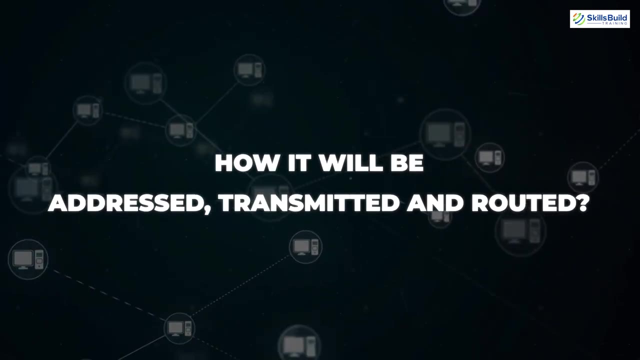 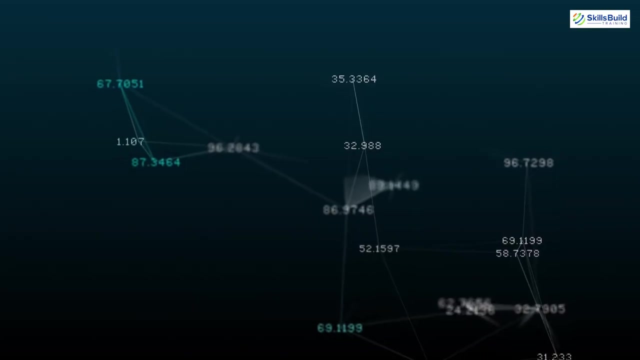 and it provides end-to-end communication to make sure that your data gets transferred successfully and, with the help of end-to-end communication, it identifies that how the data will get broken into packets then how it will be addressed, transmitted, routed over the network and how it will be received at the destination. if we say the main emphasis of tcp ip is to ensure 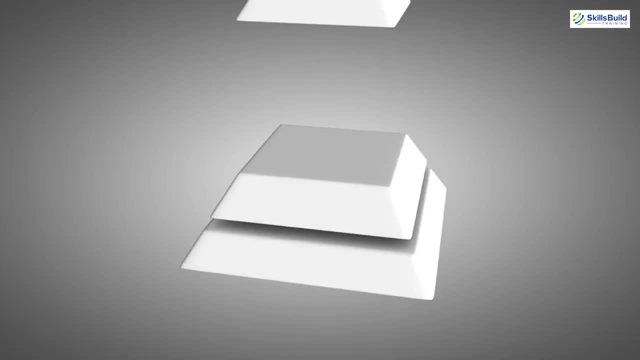 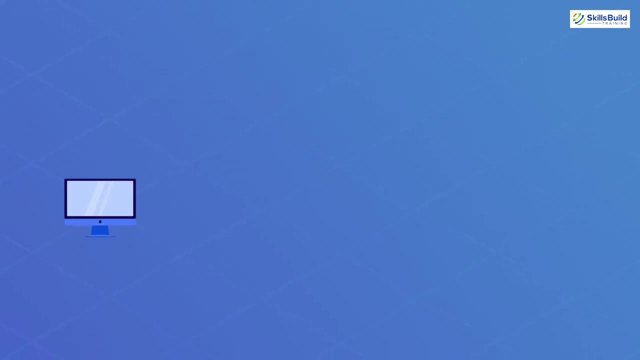 and maximize the accuracy. it would not be wrong to make sure that it gets the accuracy. there are a lot of steps involved in it. imagine if the system sends the message or data as a single piece and on the way to its destination the message or data gets lost. now what would the network do? 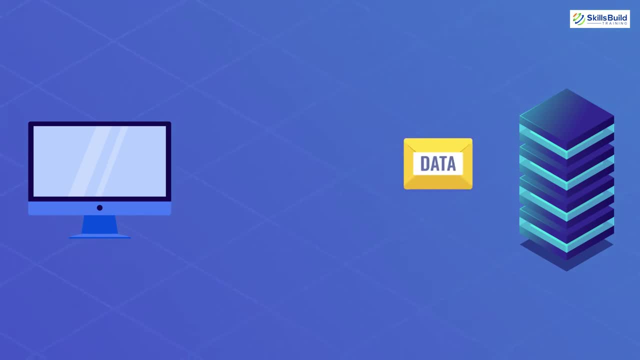 obviously it will have to send the data again, but that can cause a lot of delay in the data transmission and along with that, the data will consume a lot of resources from the network, as it will be sending a lot of data to the network and it will be sending a lot of data to the network. 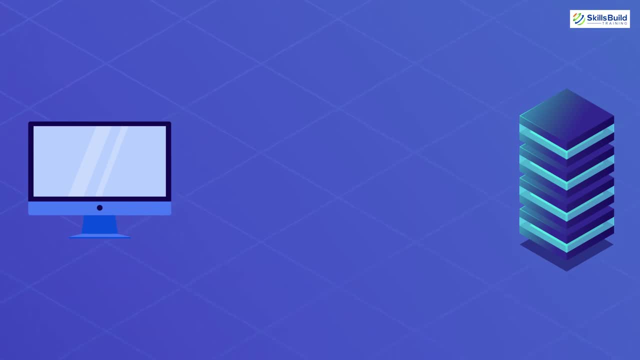 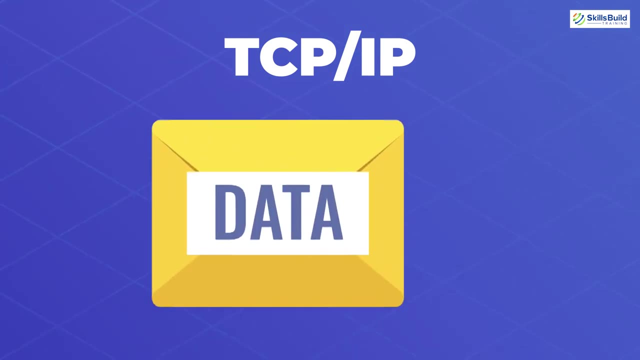 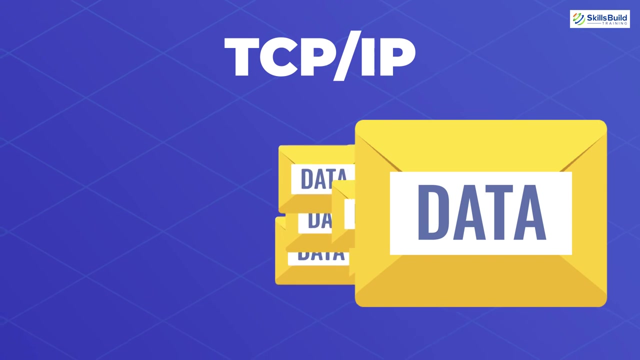 the data again and again in case of data loss. but with the help of tcp ip we get to solve this problem, as i have talked earlier when i was talking about the osi layers- that our messages get divided into segments and then those segments gets divided into packets. tcp ip breaks the data. 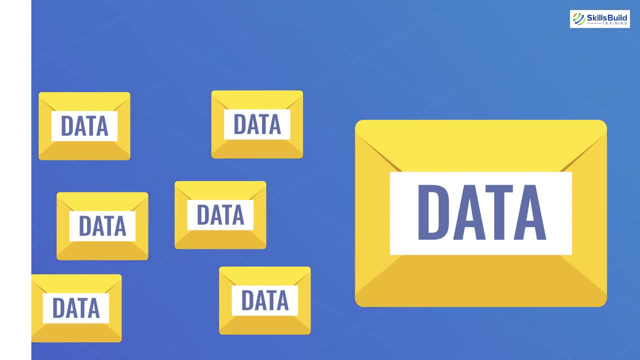 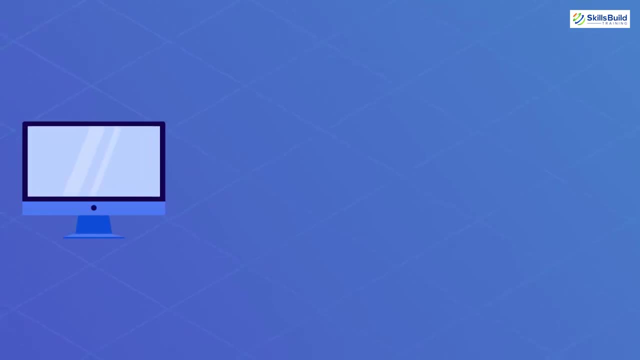 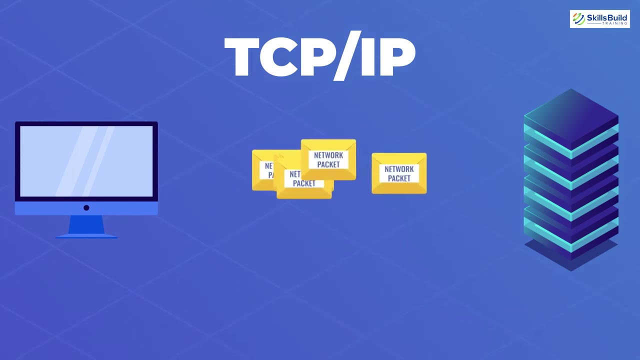 or message into packets. once all the packets reach the destination, all are reassembled again. now what is the benefit of converting our data or message into packets? the answer is really simple. in case if any of our packets of the data gets lost during the transmission, the network does not have to send the whole data or message again. 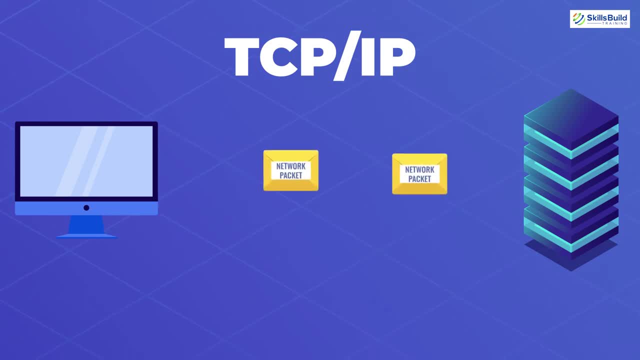 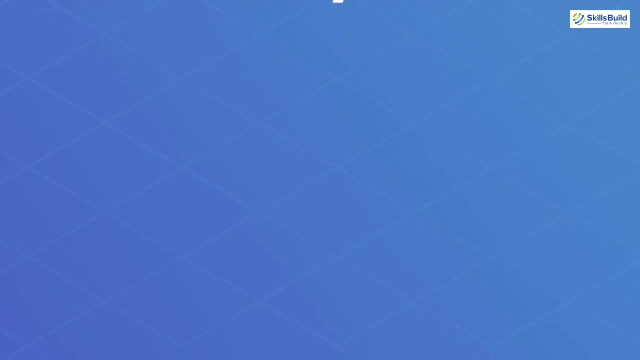 it just needs to send the lost packet and because of that the data and messages gets transferred to yourvenidos to the network more quickly and it will consume fewer resources as compared to when the network had to send the whole data again. tcp ip uses the four layers for communication. 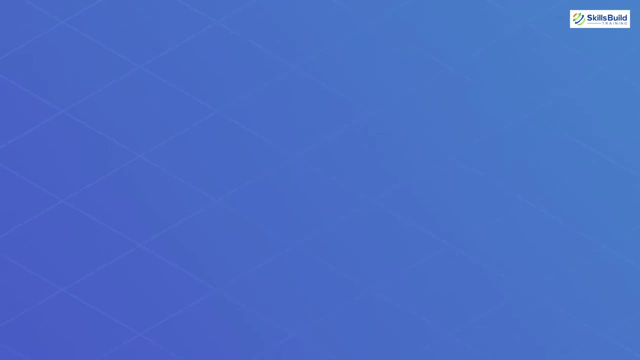 tasks and each layer has a different function. the first one is the data link clear. it is also known as the link layer and in some networking model it is also known as the physical layer. this layer is responsible for the handling of the data and all economic편ientes of the data network. it will not need monthly connections to be ableUTип using data.